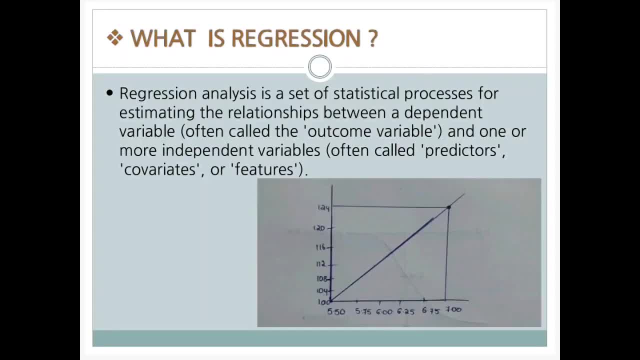 video. Before going to know what is logistic regression, first of all we need to know what is regression. Regression analysis is a predictive modeling technique. It estimates the relationship between a dependent and an independent variable. What is dependent variable and what is independent variable? Dependent variable is nothing but. 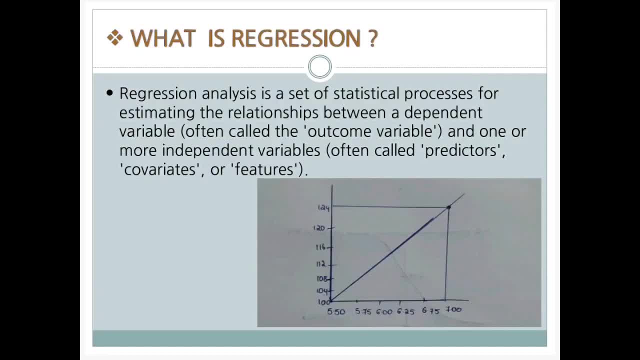 which I want to predict Now. let's say I want to know what will be the sales on 17th of this month. Then sales becomes a dependent variable or target variable. this dependent variable or target variable is going to depend on lot of factors, suppose let's. 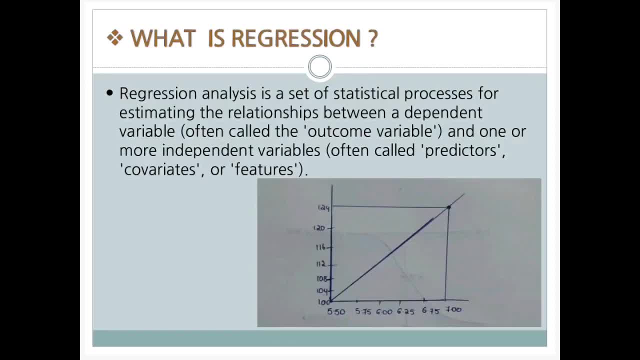 say the number of products you sell till late, or in which season you sold. is there any availability of product or product quality? all these things are the factors, so these are never ending factors. so these variables are called as independent variables. it can be better understood through a graph. suppose, if we consider a graph, if we see this graph, as the x value increases. 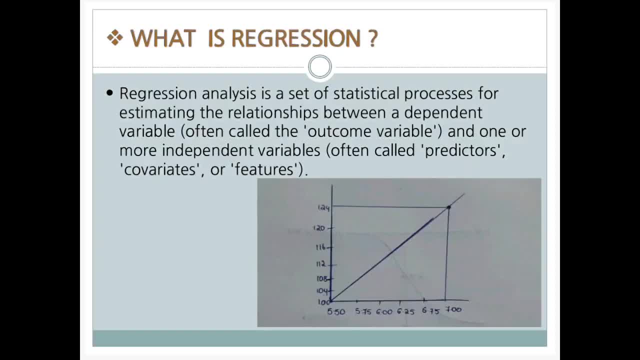 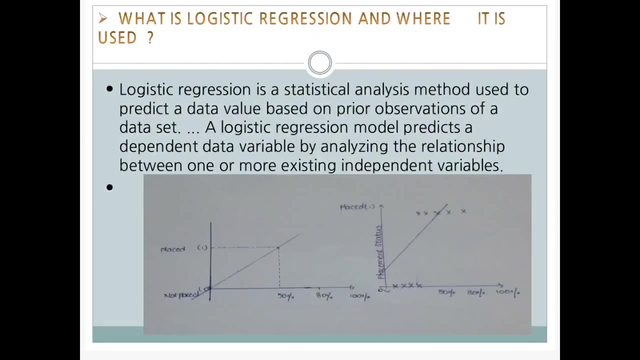 then the y value also increases. suppose our data point is at 6. then someone asks you: what? what is the value of y here we can use? we can predict the answer through fitting a straight line. i think you have understood what is regression. now we shall discuss about logistic regression. 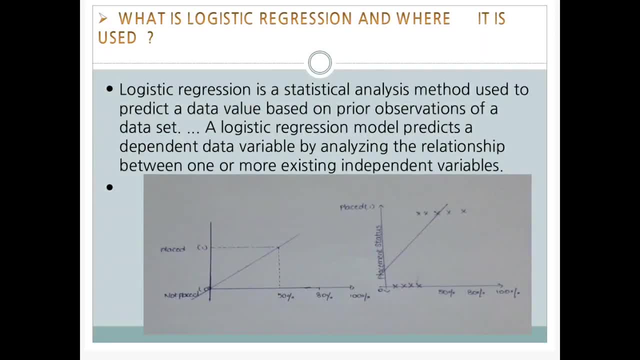 first of all, what is logistic regression and where it is used? logistic regression is used in classification problems where the labels are discrete number of classes, as compared to linear regression, where labels are continuous variables. this type of algorithm is used when output is in binary format, that is, it is used to predict. 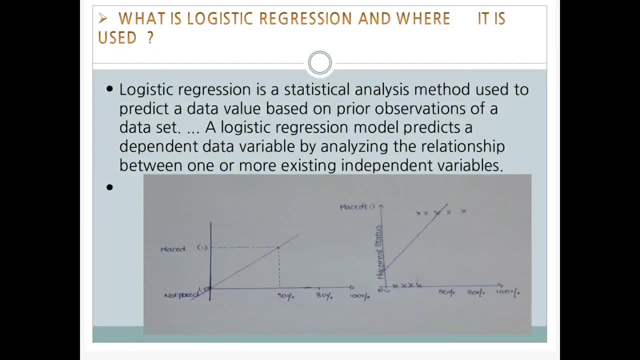 the outcome of a categorical dependent variable. so outcome be such as yes or no, high or low, place your not, place zero or one, the value should be discrete, categorical. you can have a doubt: why can't we use linear regression in case of logistic regression? and the answer is: 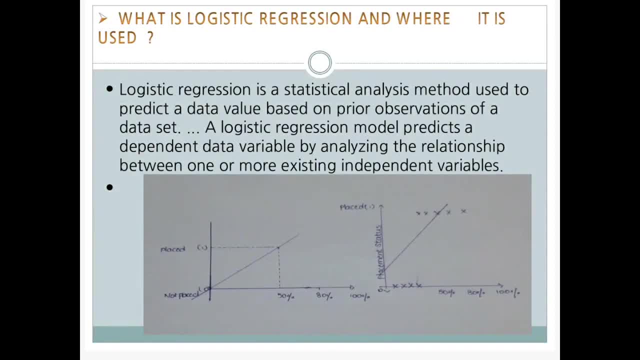 no, because linear is used to predict in a range, whereas logistic is used to predict only two values, either 0 or 1. it could be better understand by taking an example. suppose if we consider student placement data set for now let's consider lesson that would be congratulate to use either of. 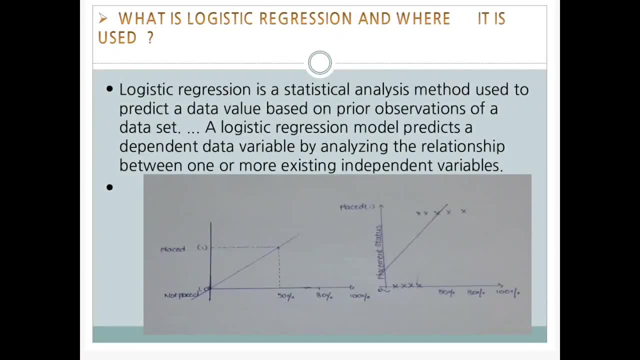 представ. the placement status of students is only based on BTEC percentage and if we try to fit a line, we can notice that people having BTEC more than 50% are getting placed. and now consider the below data: where student has, approximately 93% is added to the data. If you try to fit a line now, we can. 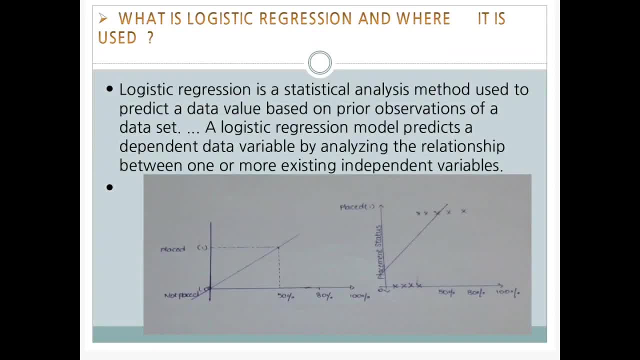 see that people are wrongly classified. in fact, linear regression doesn't seem to work well in the case of discrete attributes. This sensitivity to outliners is one reason. linear regression is a poor choice for classification problems. In classification we want the class label to be 0 or 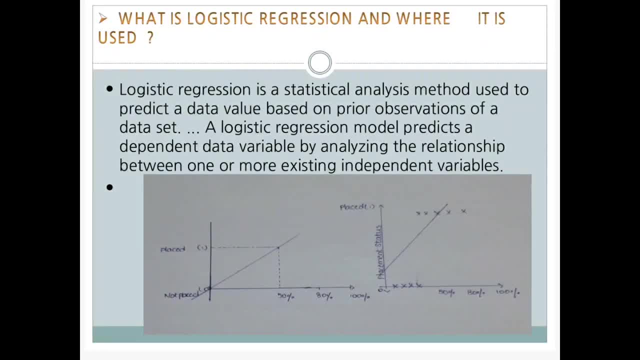 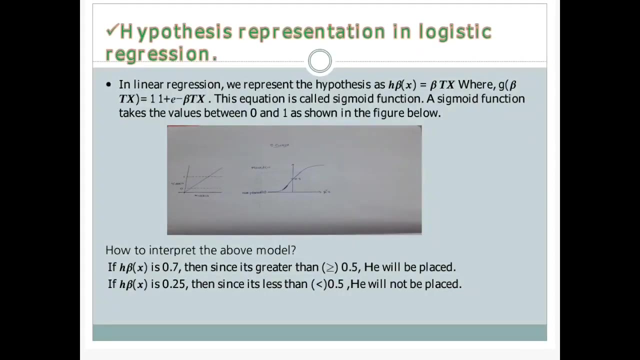 1, but in case of linear regression we take a value greater than 1 or less than 0, so we need to convert the linear regression in the way we have the values only in between 0 and 1.. In linear regression we represent the. 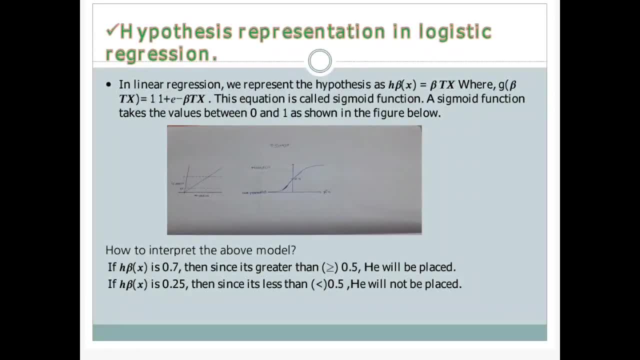 hypothesis: SH beta of x is equals to beta power t into x, where g of beta t x is equals to 1 by 1 plus e power, minus beta t into x. This equation is called a sigmoid function. A sigmoid function takes the values between 0 and 1.. This is an S curve sigmoid function curve. The sigmoid basically converts any value from minus infinity to plus infinity, to a discrete value. 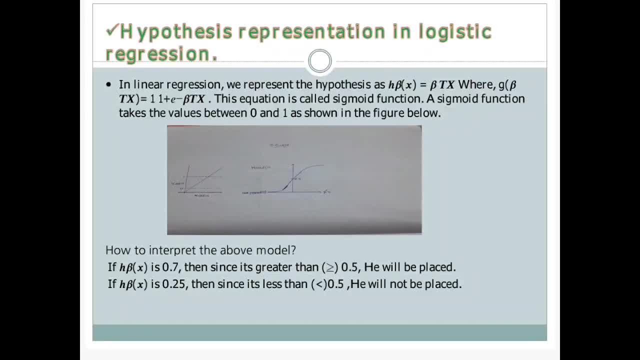 Which logistic regression wants. that is, either 0 or 1.. To understand more about it we should consider a graph. In the graph, suppose our point is 0.8. then we need to decide whether our answer is either 0 or 1.. Then how to decide it? Now, here we can use the concept of threshold, which 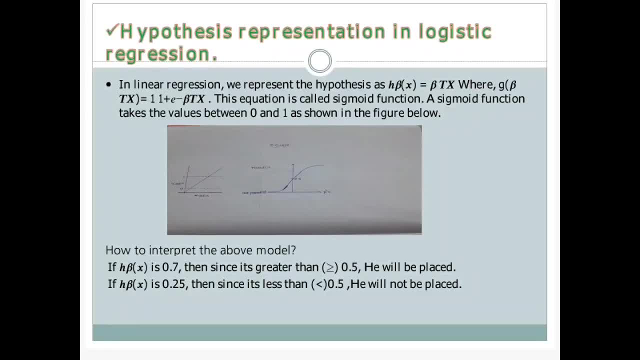 basically divides the line. Threshold value indicates the probability of either winning or losing. value equals to one. losing means equals to zero. now we can check how it works. suppose our point is a 0.8, then we need to check whether our point is above the threshold or below the threshold. 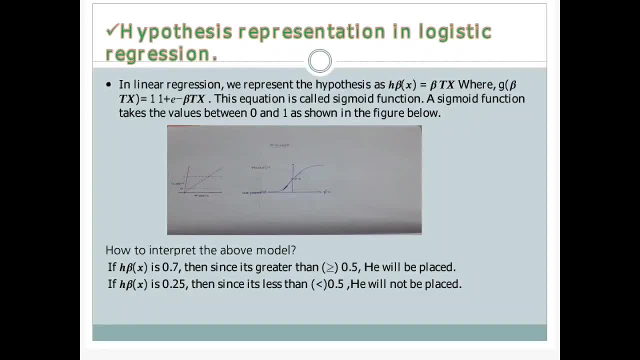 suppose if it is more than a threshold value, then it gives a result as one else gives result as zero. suppose we think threshold is 0.5, then we need to know whether our value is more than 0.5 or less than 0.5. if it is more than 0.5, then it is win, so it is one, or else if it is less than 0.5, 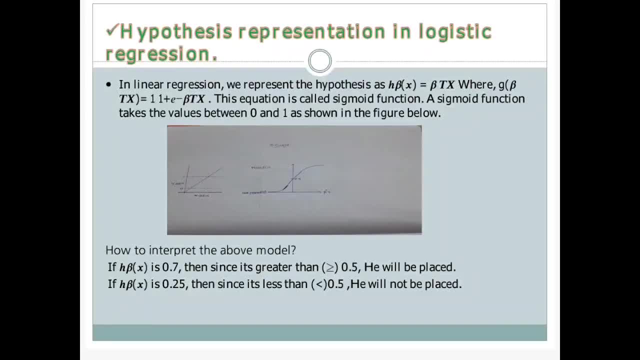 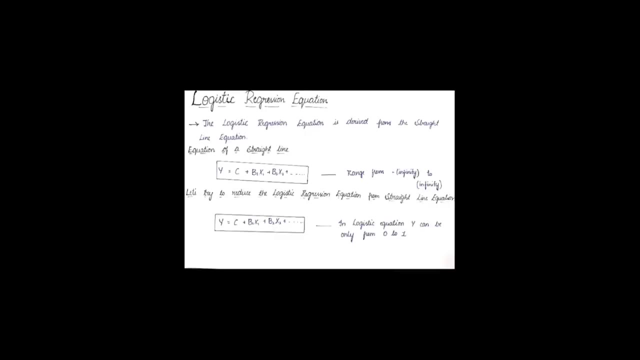 it is zero lose. we can. so we can use this concept to know better about logistic rig. this is sigmoid curve. hello friends, my name is mercy and i am from csc department. now let's see how an equation is formed over here. we have an equation of a. 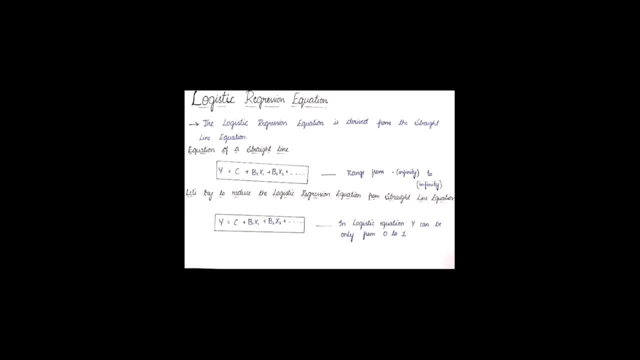 stratigraphy line, which is y, is equal to mx plus c. so in this case i just have only one independent variable. but let's see, if you have many independent variables, then the equation becomes m1, x1 plus m2, x2 plus m3, x3, so on till m and xn. so let us put in b and x. so here the equation becomes: 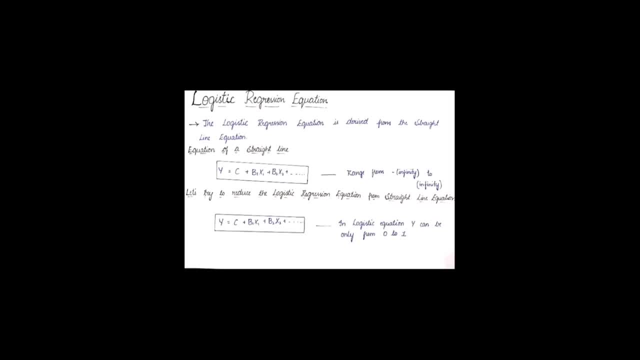 y is equal to c plus b1, x1 plus b2, x2 plus b3, x3 plus, so on till b and xn. the equation of a straight line has a range from minus infinity to infinity, but in logistic equation the value that means which we need to predict it, can have the 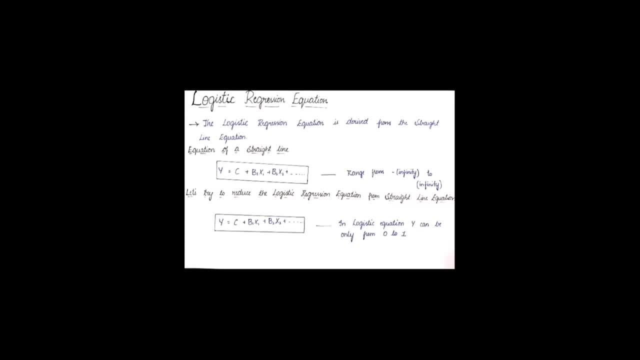 range only from 0 to 1. so in that case we need to transform this equation. so to do that, we had divide the equation by 1 minus y. now if we take y is equal to 0, we get, and if you take y is equal to 1, then we get infinity. Now, here the range is from 0 to infinity. 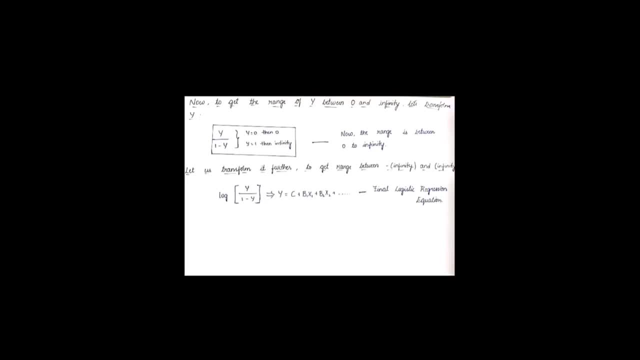 but again, if we want range from minus infinity to infinity, So for that we have to apply log for this equation. So let us transform it further to get range between minus infinity to infinity. Here we have log over y by 1 minus y, then we get the final logistic regression equation. 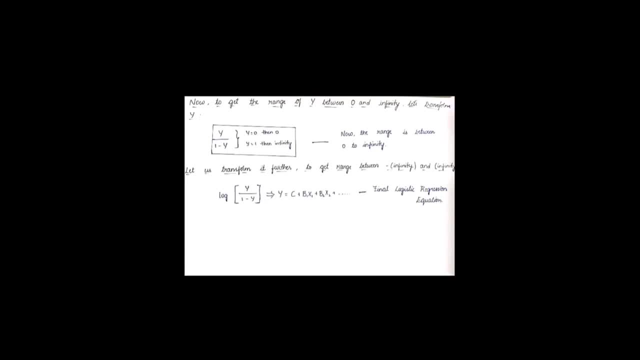 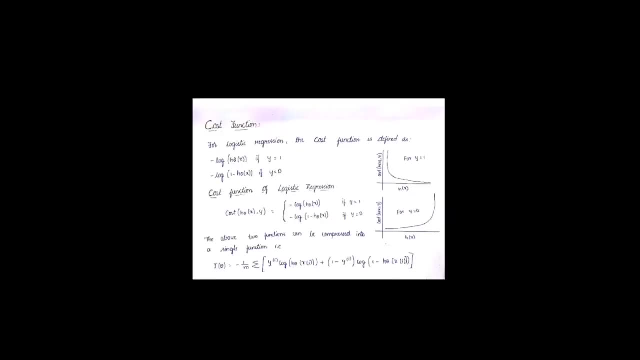 which is y, is equal to c plus b1, x1 plus b2, x2 plus so on. Now, coming to the cost function. the cost function represents optimization objective, that is, we create a cost function and minimize it so that we can develop an accurate model with minimum. 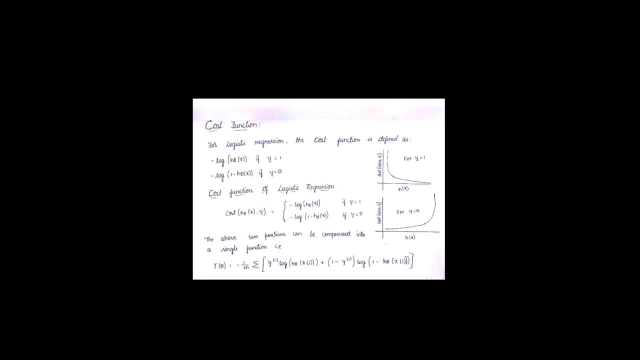 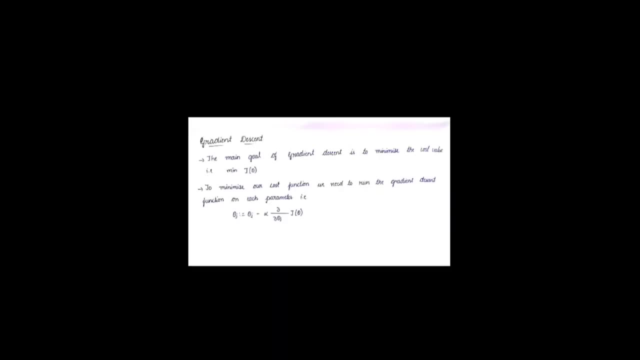 error. Here you can see how the cost function is defined. So the two functions compressed into one cost function. Now the question arises that how do we reduce cost value? Well, this can be done by using gradient descent. The main goal of gradient descent is to minimize the cost value. 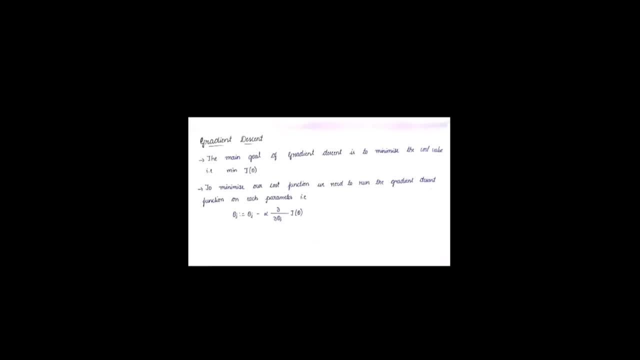 Now, to minimize our cost function, we need to run the gradient descent function on each parameter. Gradient descent has an analogy Which we have to imagine ourselves: at the top of the mountain valley and left stranded and blindfolded. Our objective is to reach the bottom of the hill, Feeling the slope. 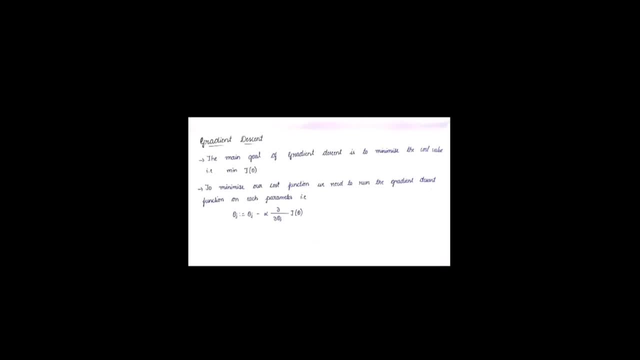 of the terrain around you is what everyone would do. Well, this action is analogous to calculating the gradient descent, and taking a step is analogous to one iteration of the update to the parameters. Now let us see various use cases in logistic regression. First is the weather predictions. Logistic regression helps you to predict your weather. 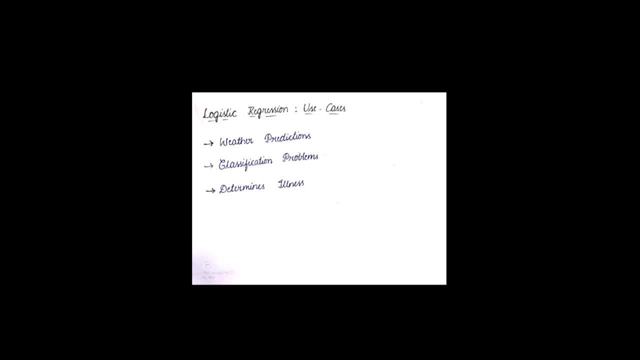 It is used to predict whether it is raining, sunny or cloudy. Now, moving to the classification problems, python performs multiclass classification. it classifies different kind of mammals in increases and decreases. deserved freedom of expression" produzca curt ret for reptiles, whether it's a reptile or not a reptile. So in logistic regression it 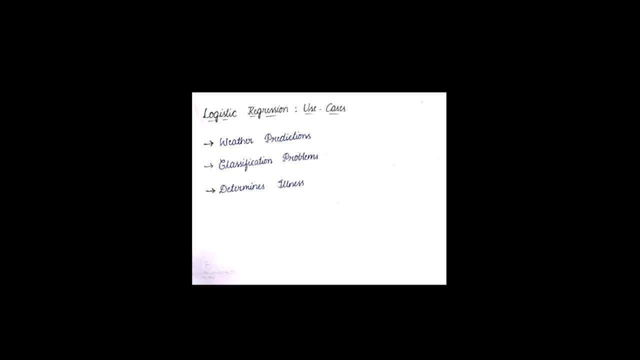 can perform multi-class classification. Next, it also helps you to determine illness as well. So let us take an example. So let's say a patient goes for a routine checkup in a hospital. So what doctor will do? They perform various tests on the patient and will. 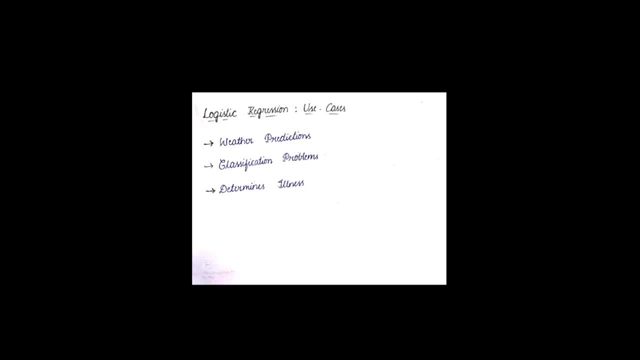 check whether the patient is ill or not. So what will be the features? The doctor can check the sugar level, the blood pressure, and what is the age of the patient, whether very small or old person, and what is the previous medical history of the patient. and 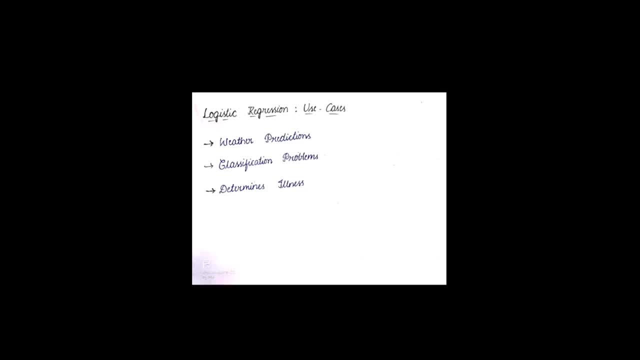 all of these features will be recorded by the doctor And finally, doctor checks the data. So, using all the data, a doctor can identify whether the patient is ill or not. So these are the various use cases in which you can use in logistic regression. 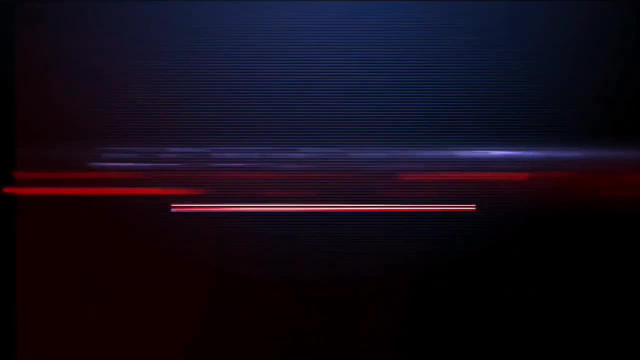 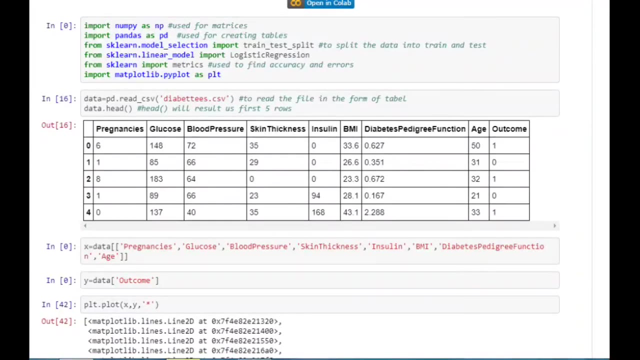 Hi friends, this is Varprasad and I am from CSC department. See the coding part of logistic regression. This is a classifier. Classification techniques are an essential part of machine learning and data mining application. Approximately 70% of problems in data science are classification problems, A popular classification technique. 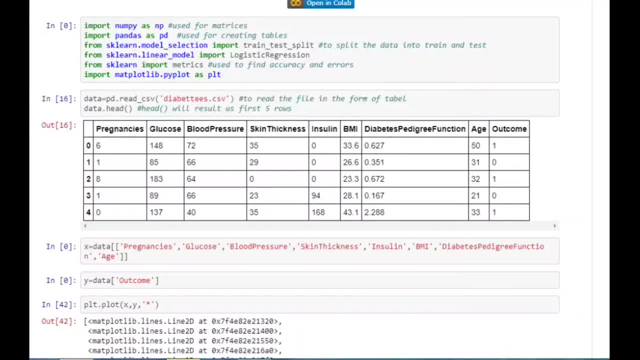 to predict binomial outcomes 0 and 1 is called logistic regression. For this we have to import all the requirement modules. Import numpy as np- This numpy module is used to create matrices and import pandas as pd. This pandas module is used to create tables For the given. 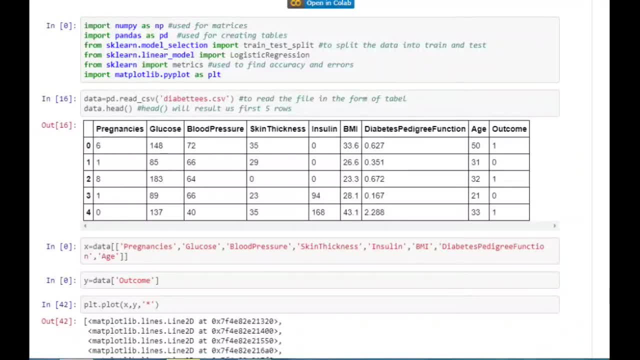 data. we have to convert the given data in the form of tables by using this pandas. From psycatlanmodel selection: import train test split. This train test split is used to split the data into train and test From psycatlan import matrices. This matrices is used to: 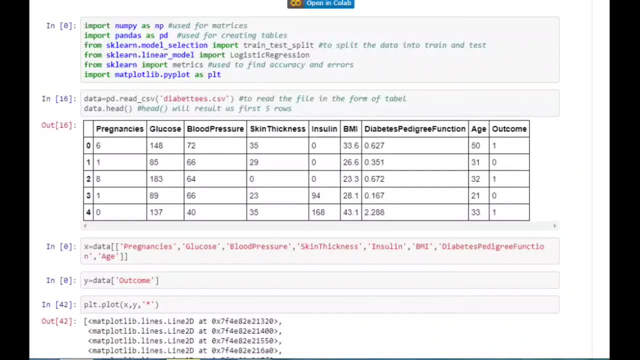 find accuracies, errors and confusion, matrix precision, etc. Import matplotlibpl by plot as plt. This is used to convert the data into graphical representation. The data remaining is diabetescsv. This is a CSV file. We are using the Increases model using index. 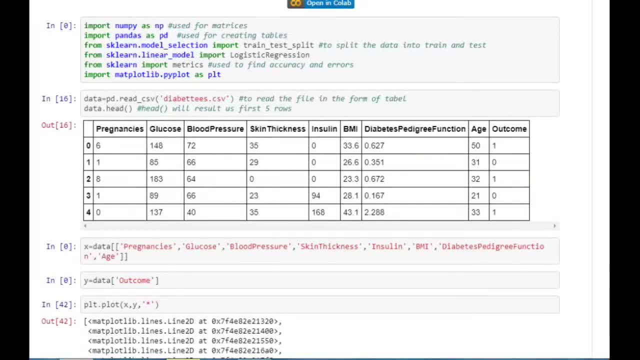 P correlation and the class label is outcome. by seeing the class label, these in the form of ones and zeros. this is a binary representation, this is a classification. so we have to divide the given data into two types of variables: dependent or target variable, and an independent variable or 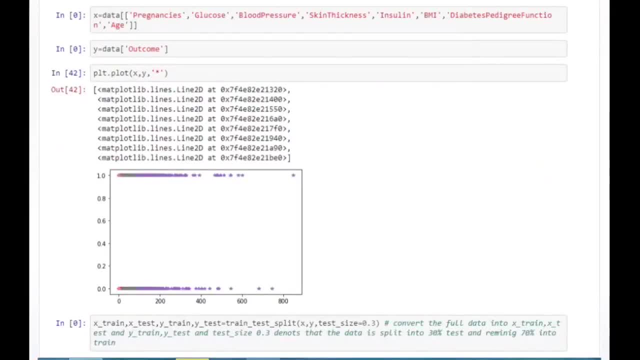 a feature variable or a class. dividing the data into two variables, we have to plot the given data. this plotting so tells us the the most of the data is near by the zero, and one more data is in between the zero and one so tells us that person does not having diabetes, and one tells just the. 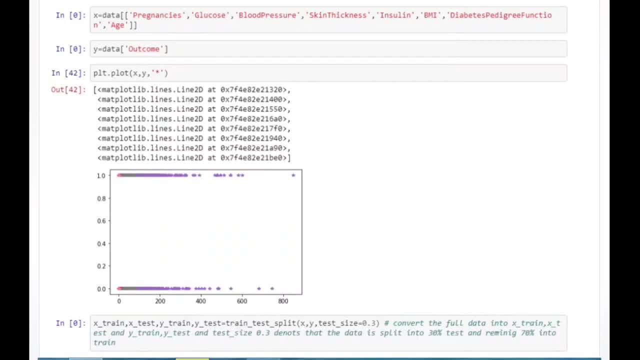 person having diabetes. by using train test split, we split the given data into two parts: seventy percent of data into training set and while thirty percent of data into test the. the test size variable is where we actually specify the property of the tests. we have given the test size as 0.3. 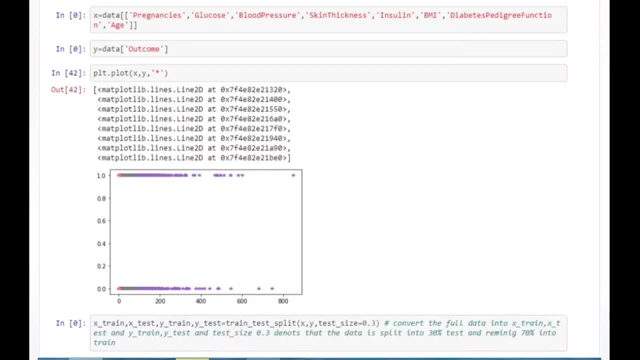 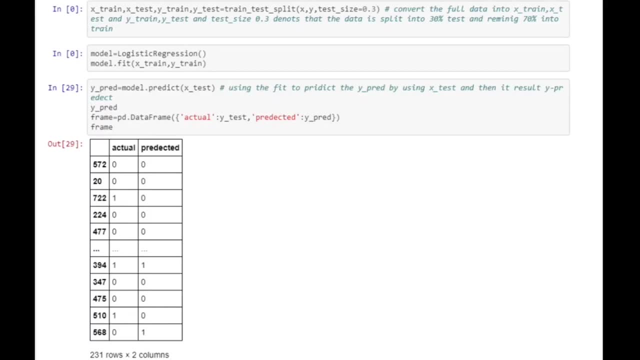 it is tells us the test size is thirty percent and the very training is seventy percent. logistic regression model using default and use fit function to train your model model is equal to logistic regression model. dot fit of x-ray and y-train. use the p, use the model by using that. 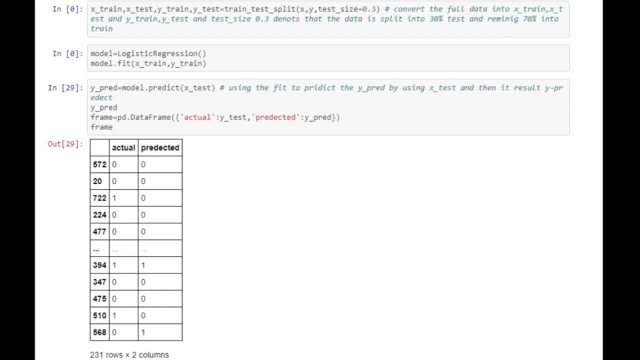 model we can predict. y-prep is equal to modelpredict of xtest. and then this x test is used to predict the y predict and we can compare the both y predict and y test. here frame is equal to pd dot data frame of y predict to predict the y predict and we can compare the both y predict and y. 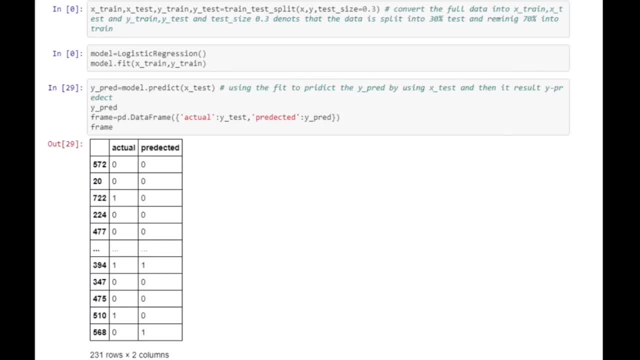 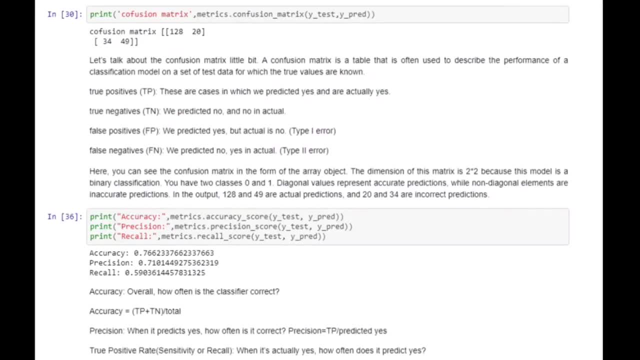 task here. frame is equal to pd, dot data frame and y-test how they are related. you can see them. let us print the confusion matrix by using this confusion matrix. this is a. this is a table that is oftenly used to describe the performance of a classification model on a set of. 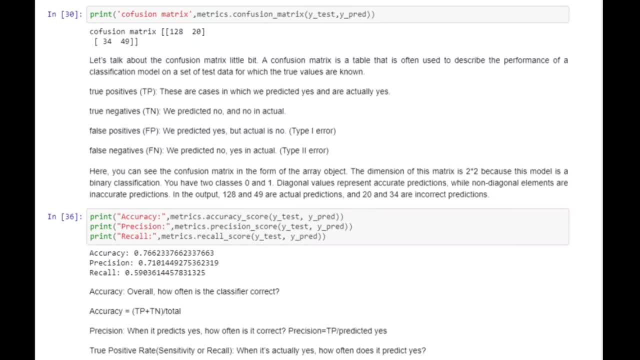 test data for which the true values are known. by using matrix module, matrix dot, confusion, matrix of y-test, y-predict, we can get the confusion matrix by seeing here: confusion matrix is 128, 20, 34, 49. this is a two by two matrix. autism metrics. there are true pause to true negative. false passé to false negative. 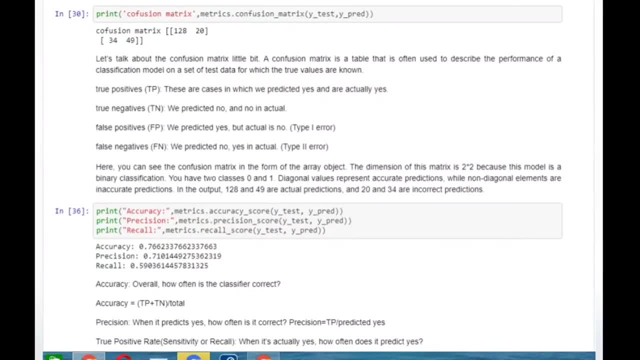 true passe to is. this is a case in which we predict yes and or actually, as I'm true- negative. we predict no under actually no. false post two: we predict test but or actually no. this is a type 1 error. and false negative. we predict no. yes, it is actually. this is type term from the. 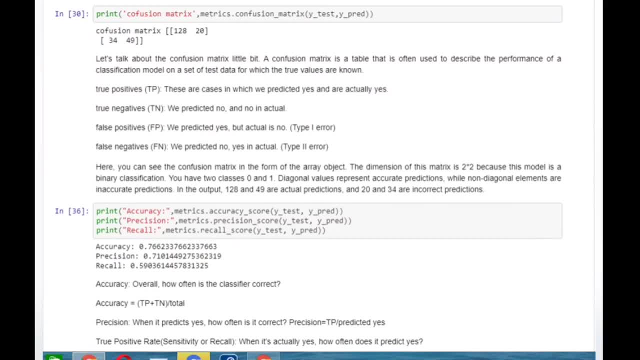 row confusion. matrix. we can see this is in the form of array object. the dimension of a matrix is 2 by 2. because this model is a binary classification, we have two classes: 0 and 1. diagonal values represent actual predictions with non-diagonal elements or inaccuracy predictions in the outcome. 128 and 49.